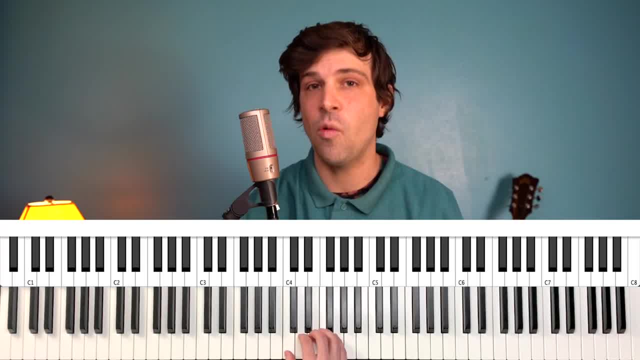 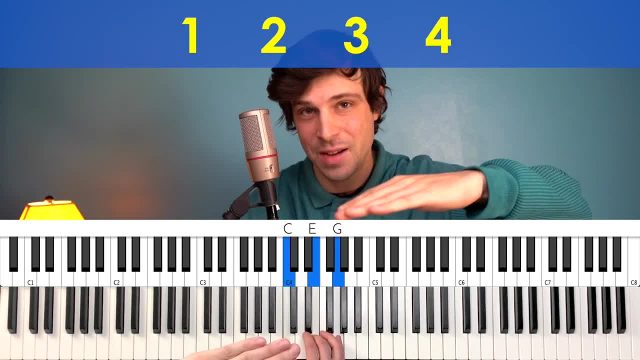 way to think about this is to be thinking in eighth notes. So if your right hand's going one, two, three, four, maybe you're tapping your foot along with those Hits. We've got to start thinking about the space in between where your foot goes up. 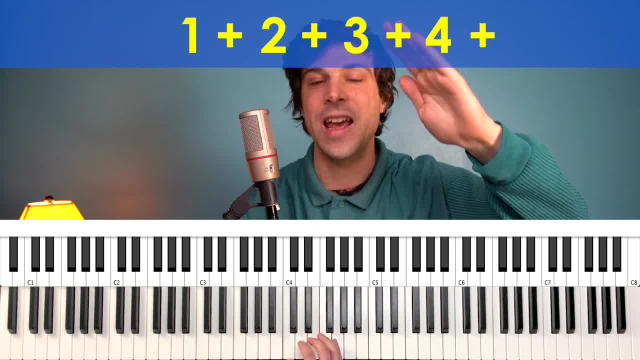 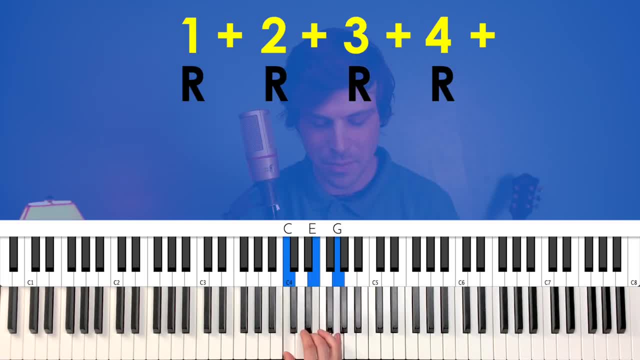 one and two and three and four, and So we're gonna put some left hand hits on those Ands. just to first get a feel for this, Do that right hand quarter note pulse. I'm just doing a C major chord. and just in between those right hand hits every single time, add a left hand low C. 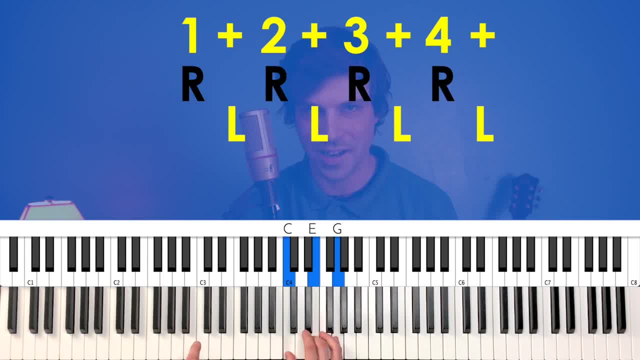 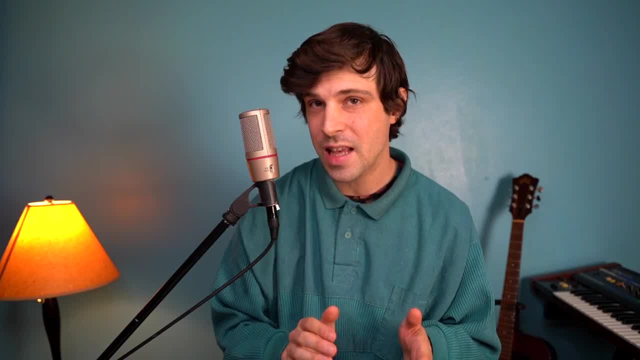 one and two and three, so you're just kind of like rocking back and forth between your hands. do that for a minute until it feels sort of natural. once you got the hang of that, we're going to thin out the left hand part to only do those alternating rhythms on the and after two. 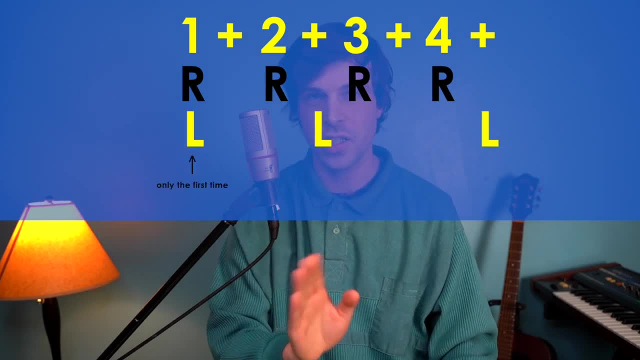 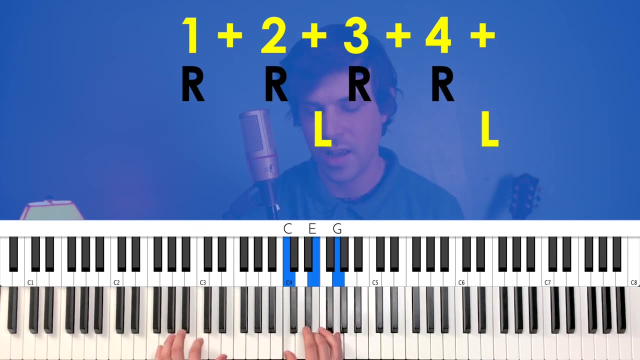 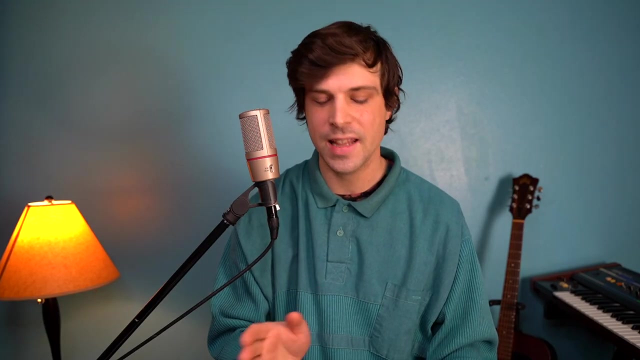 and the, and after four. we're also going to hit it once just when we start the sequence one, two and three, four, and one, two and three, four and one, two and three, four, and once you get the hang of that, you can try doing it with a chord change. so maybe let's go back and forth. 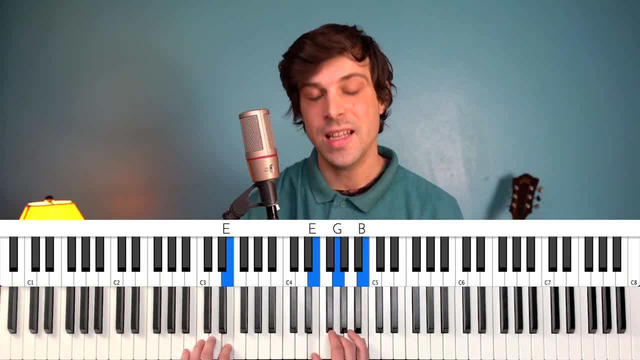 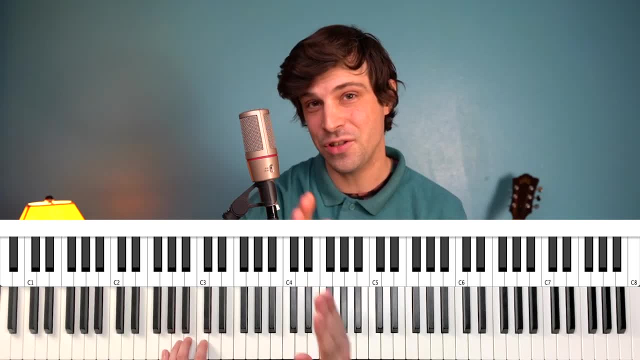 between a measure of c and then a measure of e minor. you know how, when we started that on beat one, we hit with our hands together and then from there on we were just doing the left hand on the and after two and the and after four. we're going to hit the hands together like that. 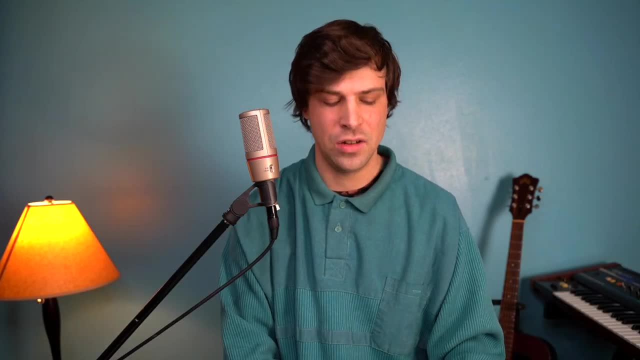 anytime you want to do that. so we're going to hit the hands together like that anytime you want to hit the hands together like that anytime you want to hit the hands together like that, anytime you want to. time you're landing on a new chord, so it's going to look like this: one, two and three, four and one. 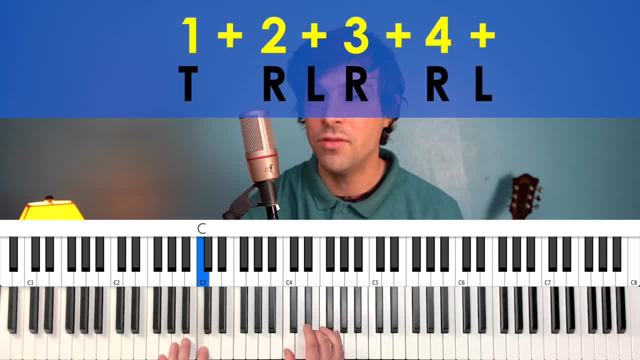 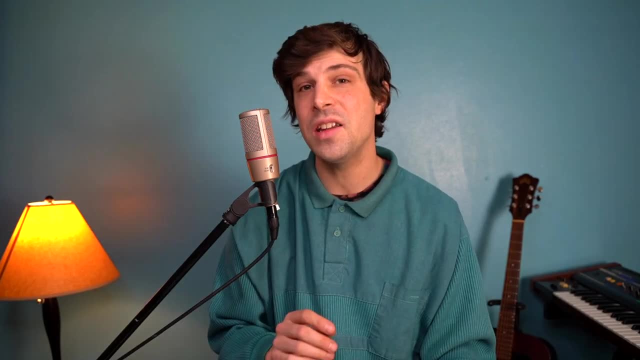 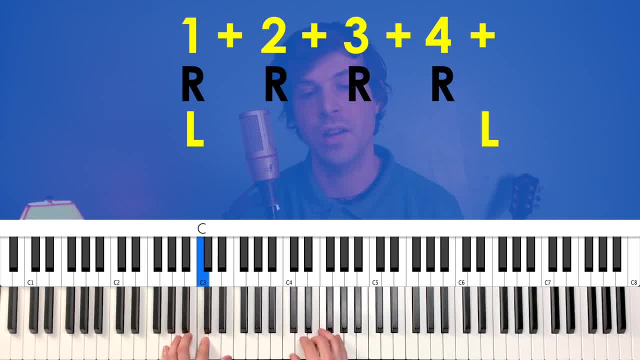 out a little bit more and only do the downbeat of the measure. and then the and after four lead out a little bit more and only do the downbeat of the measure. and then the and after four lead into the new measure, into the new measure, into the new measure. one, two, three, four and one two, three. 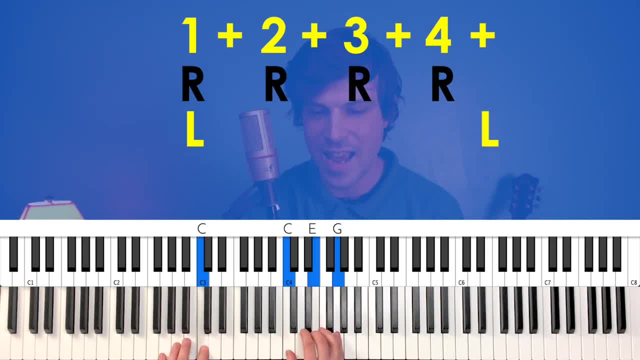 one, two, three, four and one, two, three, one, two, three, four and one, two, three, four and one. so just that. four and one, so just that. four and one, so just that. hit on the and after four kind of leads into. hit on the and after four kind of leads into. 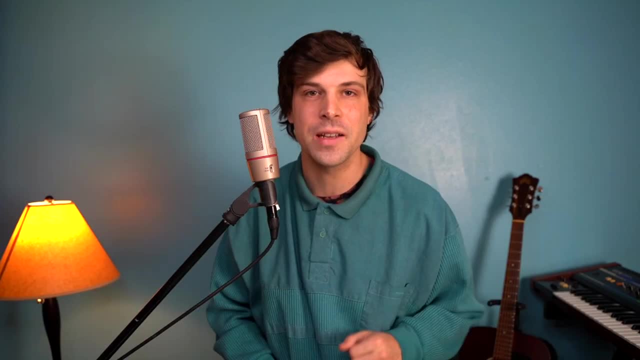 hit on the and after four kind of leads into the next chord. it just makes it feel like the next chord. it just makes it feel like the next chord. it just makes it feel like there's this forward motion happening. there's this forward motion happening. there's this forward motion happening. side note: i'm smoothing out this chord. 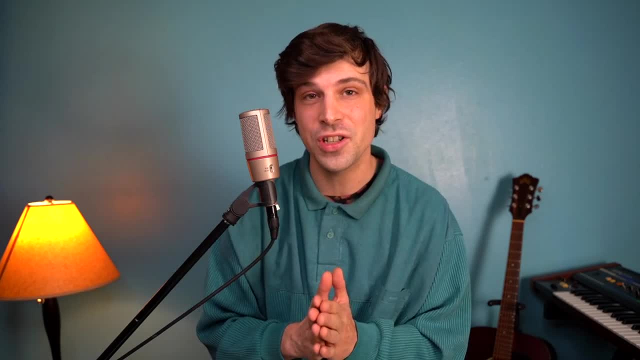 side note. i'm smoothing out this chord side note. i'm smoothing out this chord progression by holding down my sustain progression. by holding down my sustain progression by holding down my sustain pedal with little lifts every time the pedal with little lifts, every time the pedal with little lifts, every time the chord changes. check out my video on the 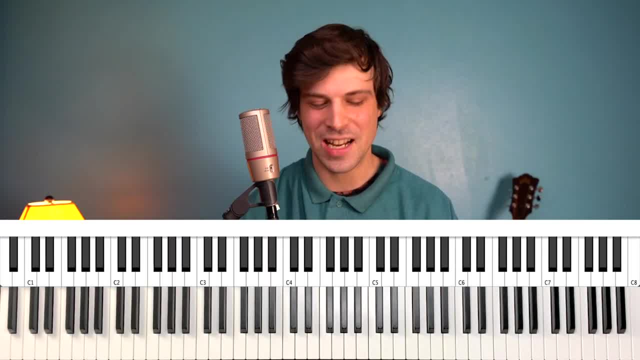 chord changes. check out my video on the chord changes. check out my video on the sustain pedal if you want to learn more sustain pedal. if you want to learn more sustain pedal, if you want to learn more. a really nice way to apply this, that. a really nice way to apply this, that. 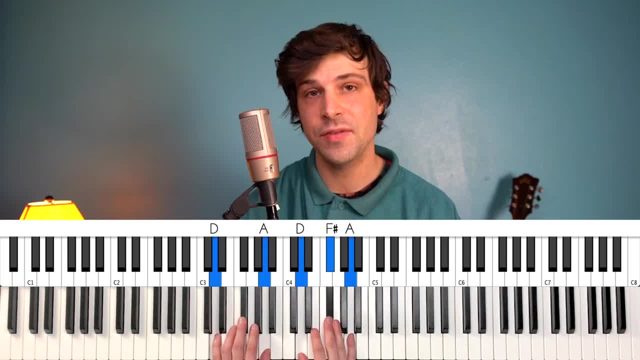 a really nice way to apply this that sounds super pretty is if you're doing sounds. super pretty is if you're doing sounds. super pretty is if you're doing fifths in the left hand, so that's like fifths in the left hand, so that's like. 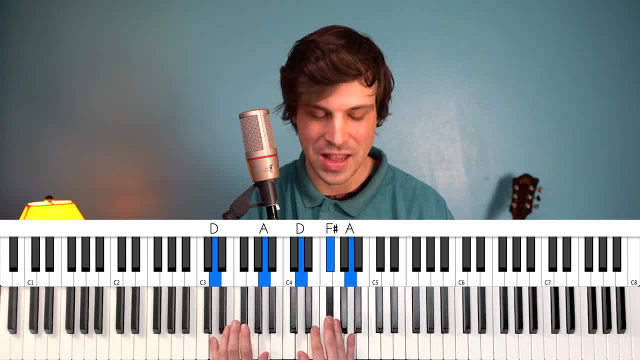 fifths in the left hand. so that's like: basically your left hand plays the same, basically your left hand plays the same, basically your left hand plays the same chord your right hand's playing, but we chord your right hand's playing, but we chord your right hand's playing, but we leave out that middle note. it's just the. 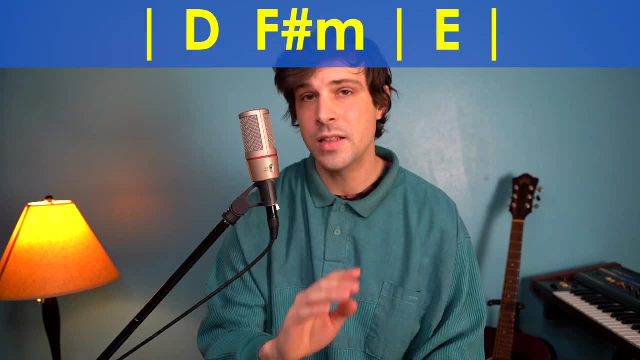 leave out that middle note. it's just the. leave out that middle note, it's just the outside notes. gives your left hand outside notes, gives your left hand outside notes, gives your left hand options for a little bit more variety. so options for a little bit more variety. so. 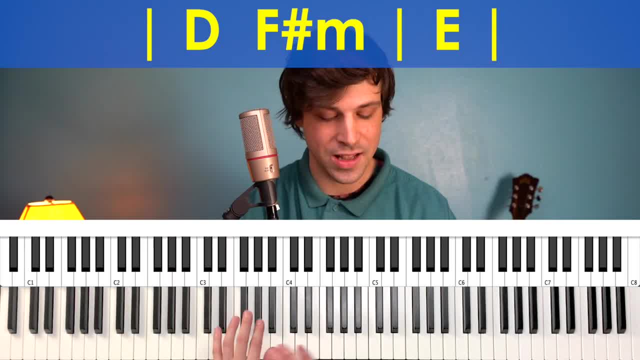 options for a little bit more variety. so let's go back to that chord progression. let's go back to that chord progression. let's go back to that chord progression. i mentioned in the beginning we're going. i mentioned in the beginning we're going. i mentioned in the beginning we're going to hit together with the fifths on one. 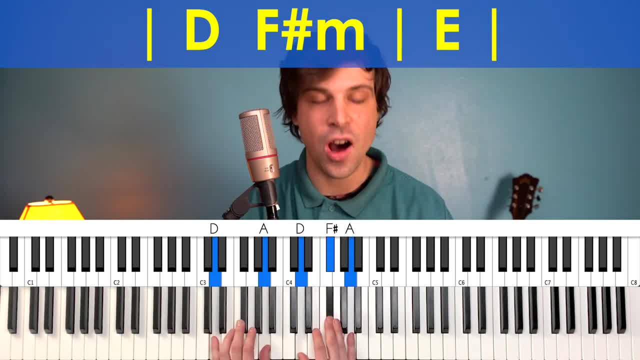 to hit, together with the fifths, on one. to hit together with the fifths on one. one, one, one, two, two, two, and. and. for that offbeat, hit the and. and. and. for that offbeat, hit the and. and. and. for that offbeat, hit the and. after two, we're just gonna do the thumb. 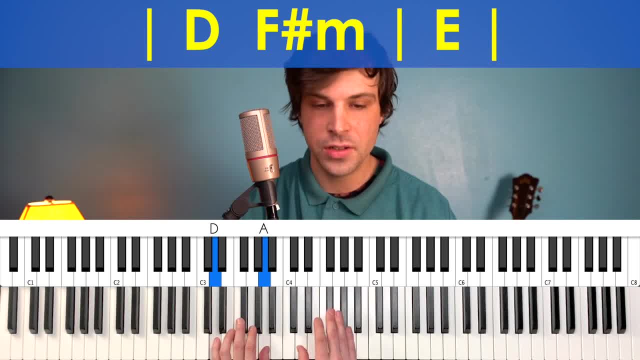 after two. we're just gonna do the thumb after two. we're just gonna do the thumb on the fifth the higher note. one on the fifth, the higher note. one on the fifth, the higher note one. two, and then we move to the new chord. two and then we move to the new chord. 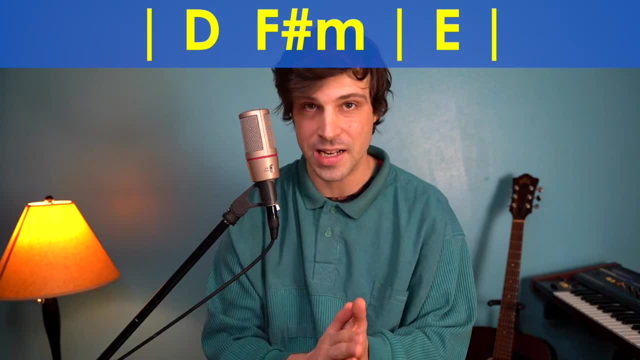 two, and then we move to the new chord. now i mentioned that rule of hitting the. now i mentioned that rule of hitting the. now i mentioned that rule of hitting the hands together. whenever you land on a hands together, whenever you land on a hands together, whenever you land on a new chord, it doesn't have to be at the. new chord. it doesn't have to be at the new chord, it doesn't have to be at the beginning of the measure. here it's in the beginning of the measure. here it's in the beginning of the measure. here it's in the middle of the measure. but we're. 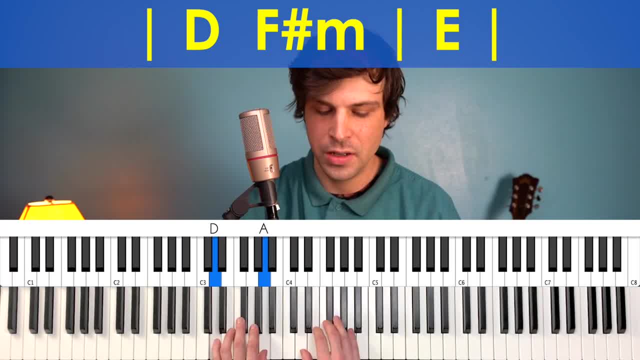 the middle of the measure, but we're the middle of the measure, but we're gonna hit the hands together on beat. gonna hit the hands together on beat. gonna hit the hands together on beat: three, one, three, one, three, one, two and three, two and three, two and three, four. and so there's that alternating. 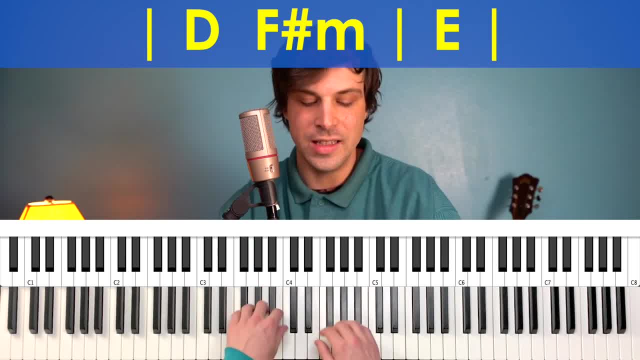 four. and so there's that alternating four. and so there's that alternating left hand hit again, where i just do the left hand hit again, where i just do the left hand hit again, where i just do the thumb leading in to the next chord, which thumb leading in to the next chord which. 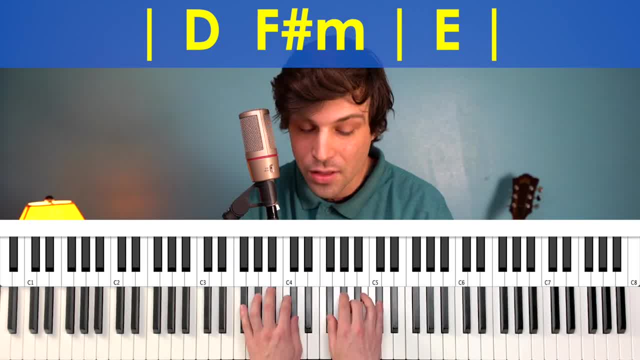 thumb leading in to the next chord, which i'm going to hit hands together one. i'm going to hit hands together one. i'm going to hit hands together one, two and three, two and three, two and three, four and one, four and one, four and one, two. now, on this e, i'm going to keep the 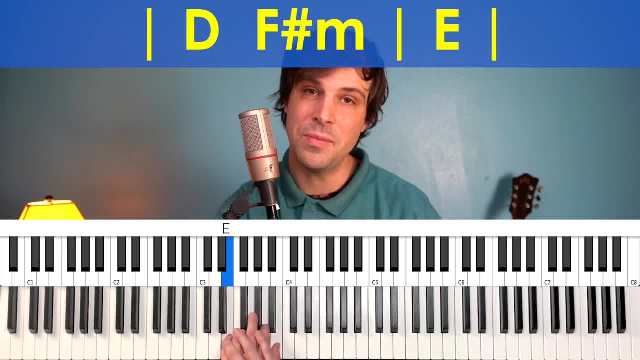 two now on this e i'm going to keep the two now on this e i'm going to keep the same rhythm going, maybe in the middle of same rhythm going, maybe in the middle of same rhythm going, maybe in the middle of this measure. i will do the bottom note. 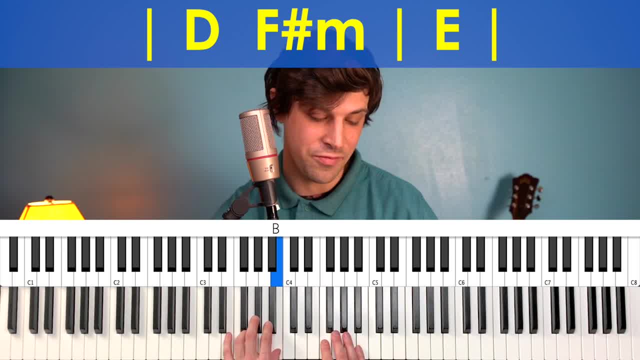 this measure, i will do the bottom note. this measure, i will do the bottom note instead of the top note, and then i'll instead of the top note, and then i'll instead of the top note, and then i'll use the top note again with the thumb. 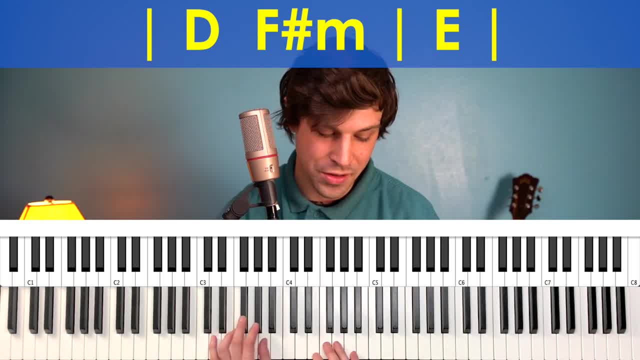 use the top note again with the thumb. use the top note again with the thumb when i'm going to lead back. so then the when i'm going to lead back. so then the when i'm going to lead back. so then the ear starts to kind of hear the, the high. 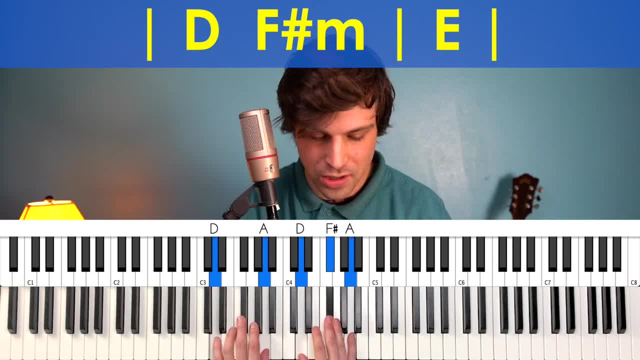 ear starts to kind of hear the. the high ear starts to kind of hear the the high note with the thumb as announcing a note with the thumb, as announcing a note with the thumb as announcing a chord change. so, chord change, so chord change. so one, two and three. 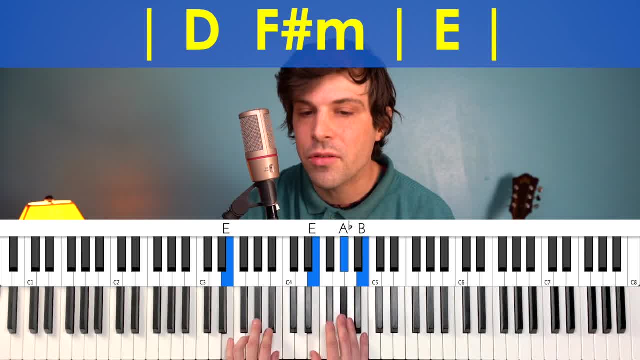 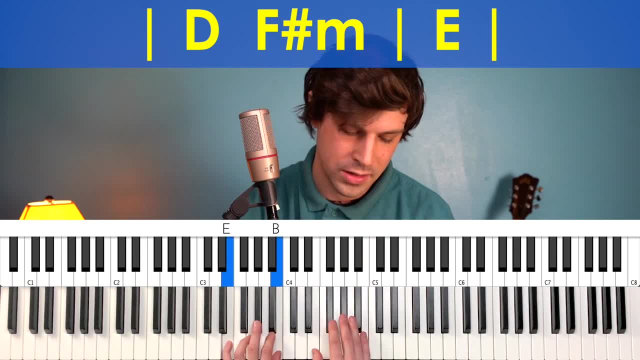 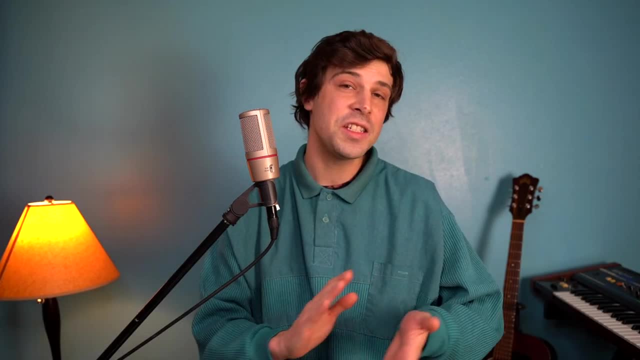 two and three, two and three, four and one just to cover all my bases. four and one just to cover all my bases. four and one just to cover all my bases here. sometimes you might be playing a here. sometimes you might be playing a here. sometimes you might be playing a chord progression that sounds just like. 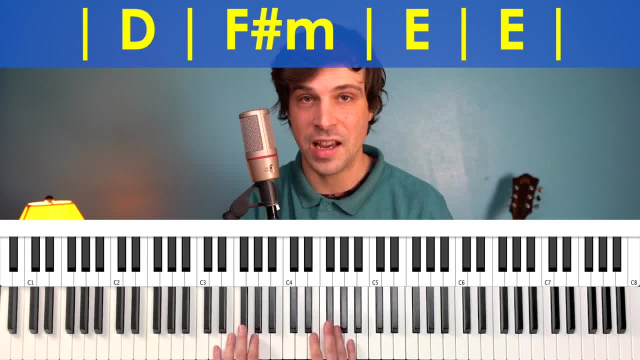 chord progression. that sounds just like chord progression. that sounds just like this. but the way you're counting it is this. but the way you're counting it is this: but the way you're counting it is in double time, so you're thinking like a in double time. so you're thinking like a. 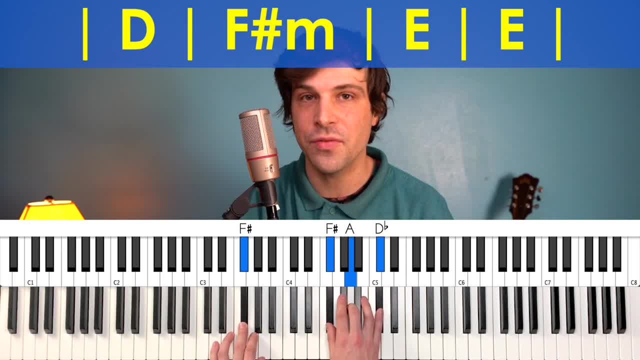 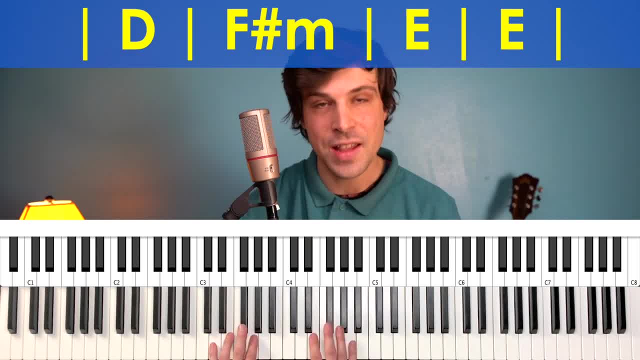 four, in which case your right hand pulse four, in which case your right hand pulse might be one, two, three, four. one in that might be one, two, three, four. one in that might be one, two, three, four, one. in that case it's actually a little easier to. 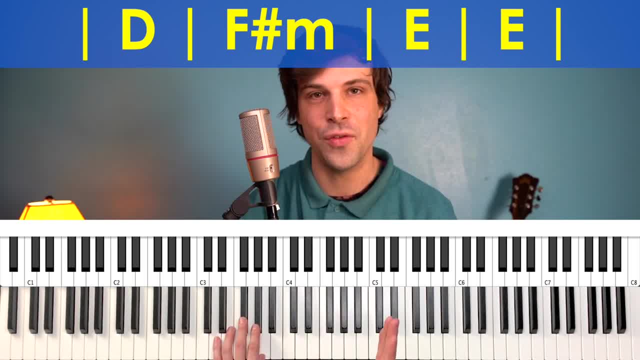 case. it's actually a little easier to case. it's actually a little easier to think about where the left hand hits. think about where the left hand hits. think about where the left hand hits, because you would hit it on one and four. because you would hit it on one and four. 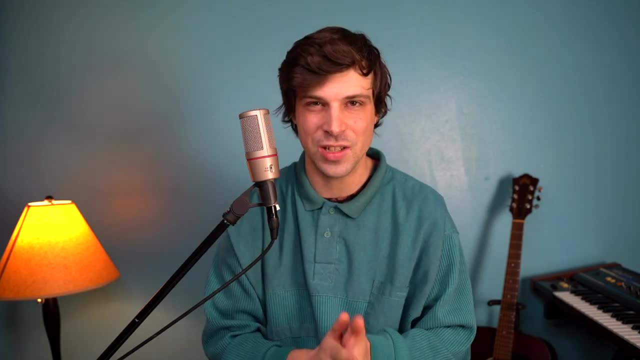 because you would hit it on one and four. you're still just whatever pulse your. you're still just whatever pulse your. you're still just whatever pulse your right hand is playing. your left hand is right hand is playing. your left hand is right hand is playing. your left hand is just playing right in the middle of. 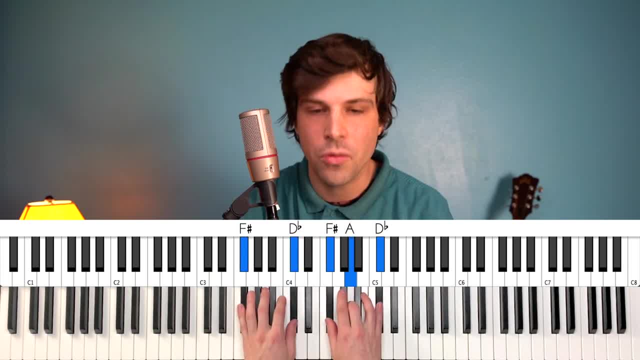 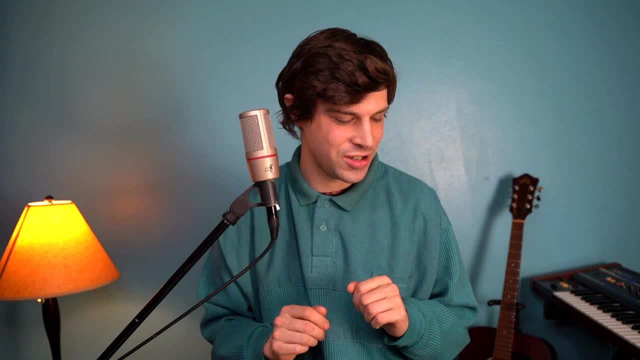 three, four one. two three, four one two, three, four one want to give one more three four one. want to give one more three, four one. two three, four, one two. example that fast and energetic one. i example that fast and energetic one. i example that fast and energetic one i showed you at the beginning. here it is. 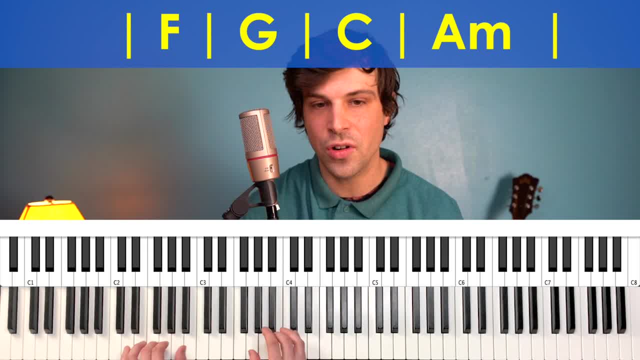 showed you at the beginning, here it is. showed you at the beginning, here it is, and we're just feeling quarter notes in and we're just feeling quarter notes in and we're just feeling quarter notes in the right hand: one, two, three, four. one. the right hand: one, two, three, four, one, two. 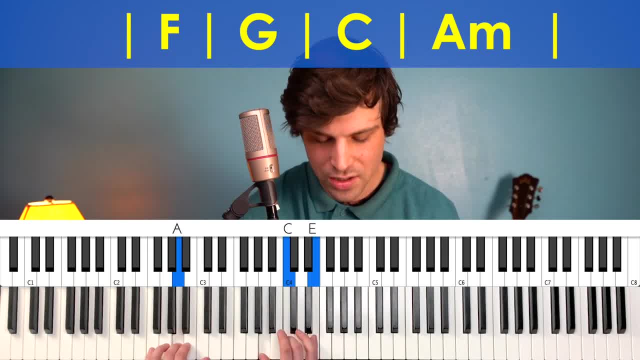 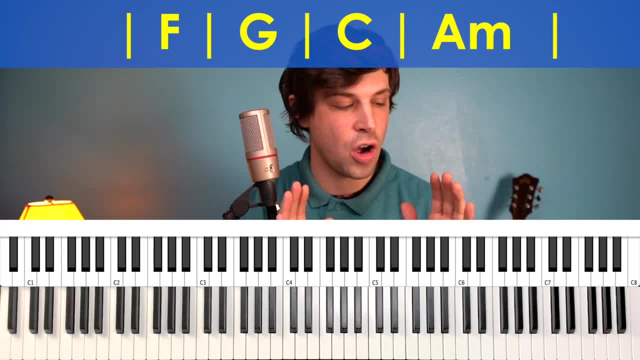 three, four, let's add those left hand hits on the and after two and the and after on the and after two and the and after on the and after two and the and after four. this time i'm going to go back to four. this time i'm going to go back to. 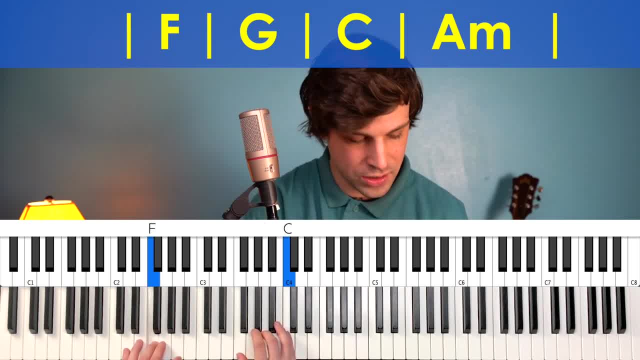 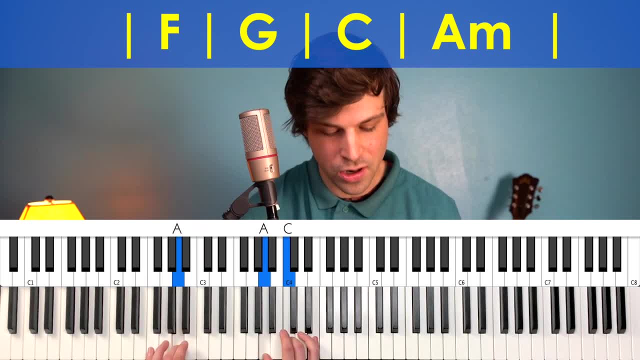 four. this time i'm going to go back to only hitting the hands together when it only hitting the hands together, when it only hitting the hands together when it lands on a new chord. try it slow if you're still getting the. try it slow if you're still getting the. 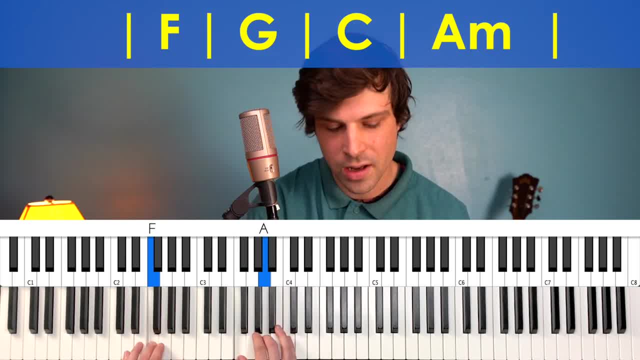 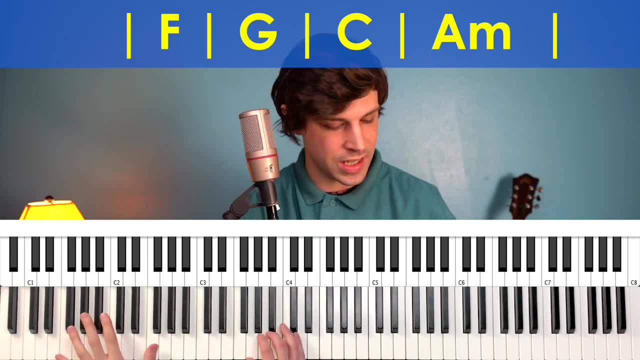 try it slow, if you're still getting the hang of this rhythm. hang of this rhythm. hang of this rhythm. one, two and three. if your hand can stretch an octave, let's. if your hand can stretch an octave, let's. if your hand can stretch an octave, let's try this. 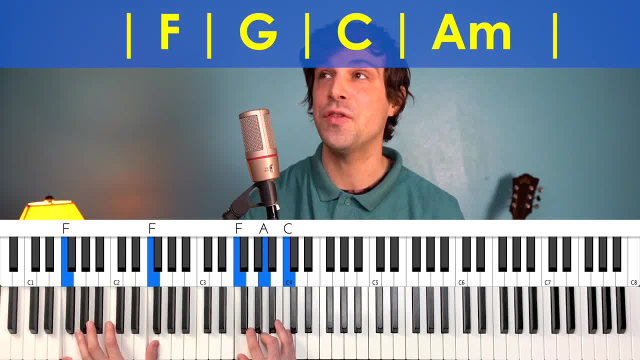 try this, try this. we're gonna do octaves in the left hand, we're gonna do octaves in the left hand, we're gonna do octaves in the left hand, and then on the, and then on the, and then on the, and, after four, the one that's leading. 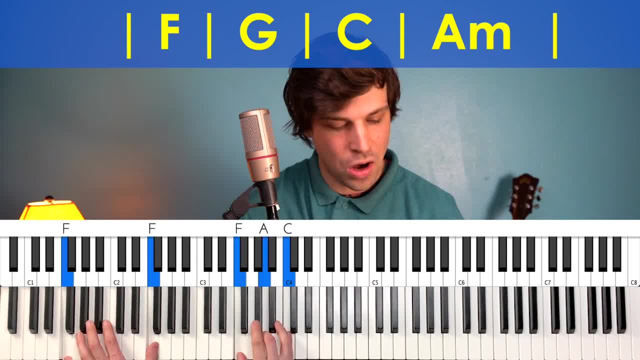 and after four, the one that's leading, and after four, the one that's leading into the new chord. i'm just gonna hit into the new chord, i'm just gonna hit into the new chord, i'm just gonna hit the top octave. just gives us some nice variety, some. 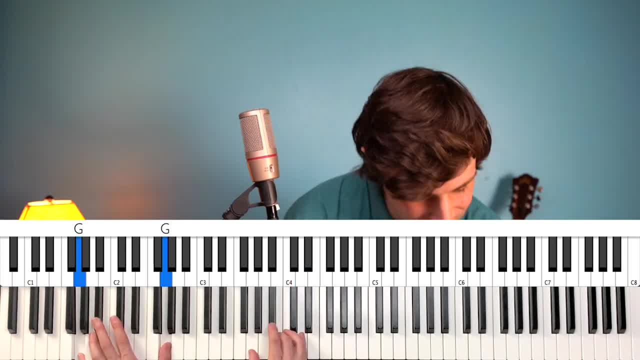 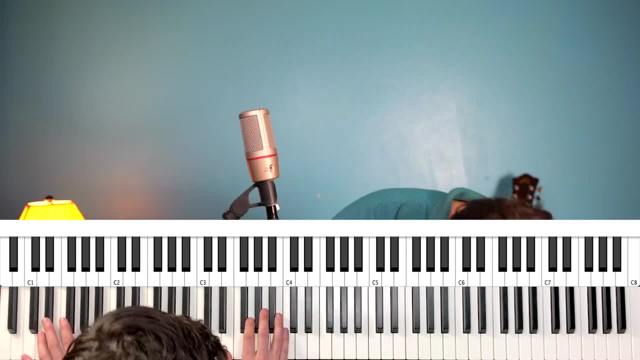 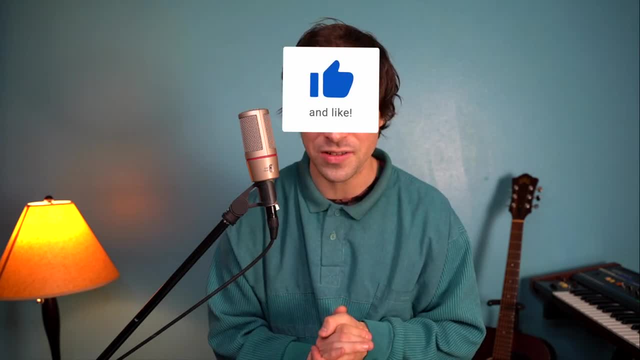 it helpful. i hope you will subscribe it helpful. i hope you will subscribe. turn on those notifications so you know. turn on those notifications so you know. turn on those notifications so you know anytime i release a new video like this. anytime i release a new video like this.